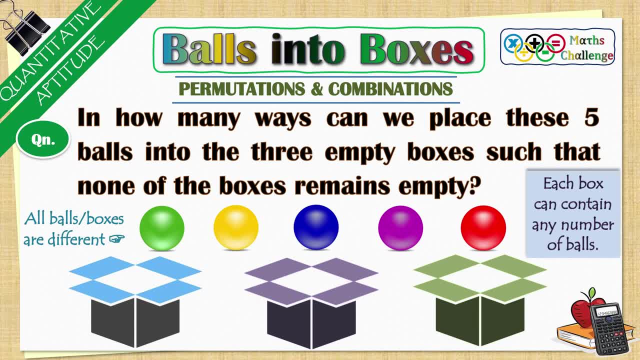 balls into the boxes such that none of the box remains empty. It's given in the question that each box can contain any number of balls. So what are you waiting for? Quickly grab a pen and a notebook and try it out, and after that we will tell you two different approaches to solve the 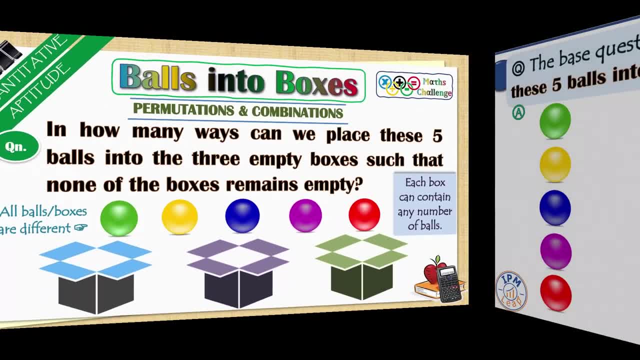 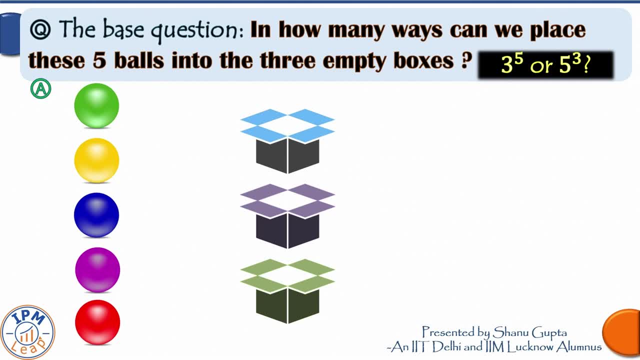 same problem. Let's begin. So, friends, before attempting the question on the title screen, first I want you to guess the answer to this space question: In how many ways can we place these five balls In this space question? we have done away with the constraint that none of the boxes should remain. 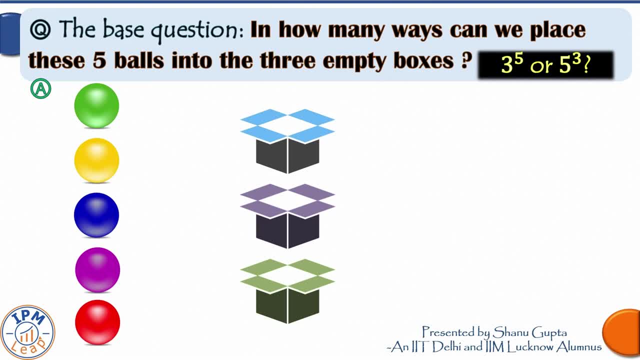 empty. This is a classic question in PNC which can be asked in so many other ways. For instance, you may be asked to post some letters into the post boxes, Or even put some coins into the pockets of your coat, And so on. It goes without saying that the 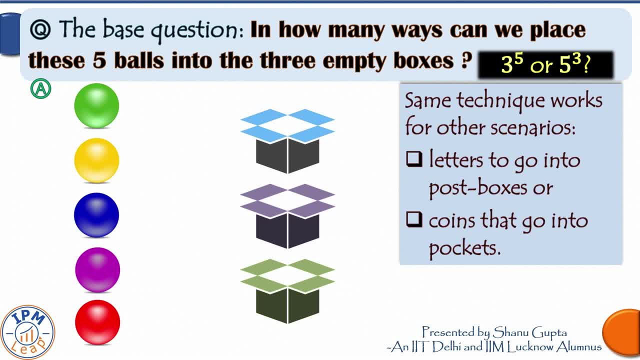 same technique that we are going to use in this question works for other scenarios as well. You have two choices for the answer: Three raised power five or five raised power three. Which one will you pick? Okay, so here is one hint which will help you in all such questions. 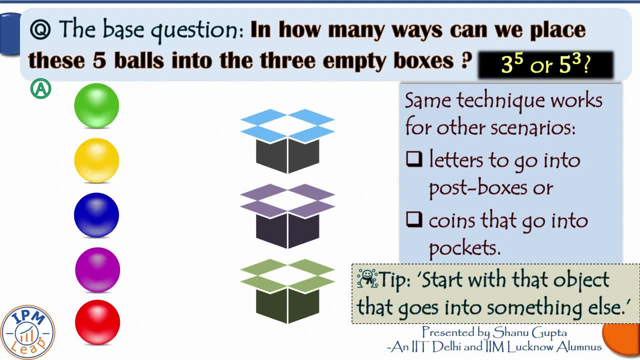 You must always, always start with the object that goes into something else, Like here in our example. balls go into boxes and not the other way around, So we start with balls. Similarly, letters go into post boxes, So we start with letters here, And coins go into pockets, So we start with coins here. Okay, 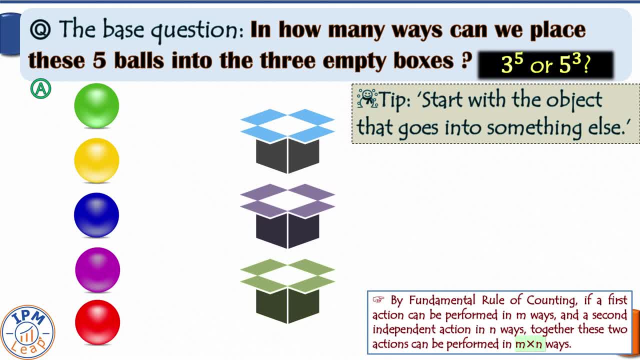 So in our case, we start with balls. Consider the number of ways in which we can place each ball, turn by turn. The first ball can be placed in three ways: into the first box, or into the second box, or into the third. Isn't it Corresponding to these three ways of? 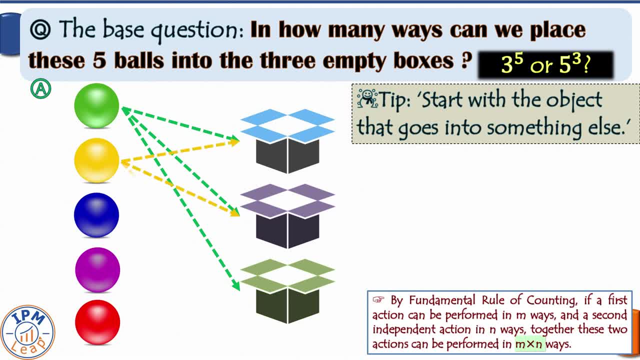 placing the first ball. the second ball can also be placed in three ways. Similarly, the third ball can be placed in three ways: The fourth in three ways And the fifth also in three ways. And remember, if you decide to place one of these balls in any, 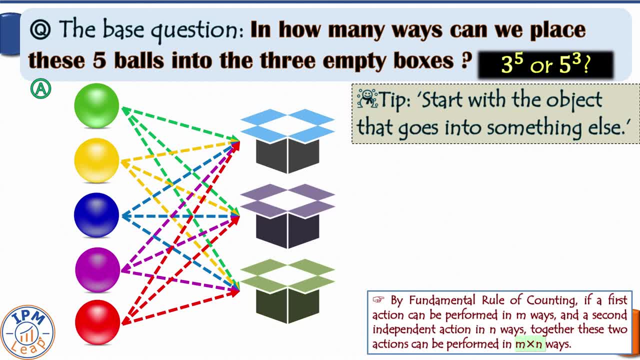 particular box. it still does not affect your options for other balls, because all boxes can contain any number of balls. For example, if I choose green box for the green ball, for the yellow ball, I again have three options, All the three boxes to choose from. In other words, 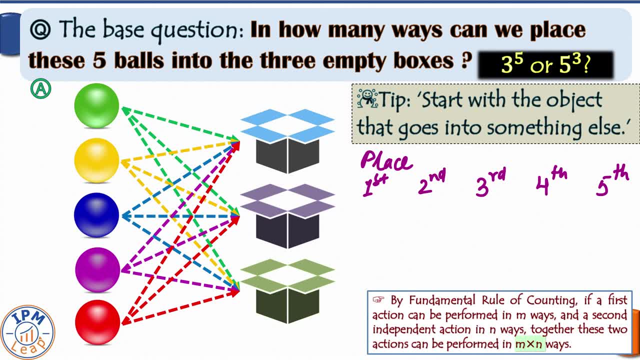 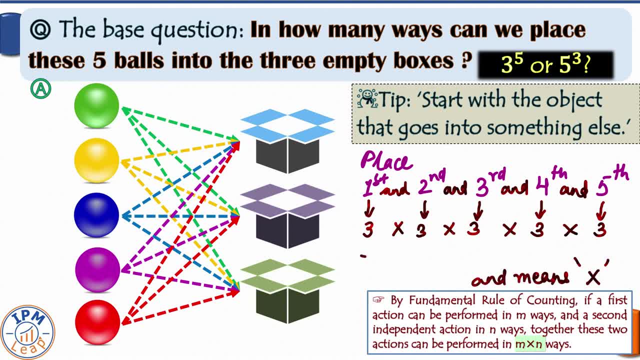 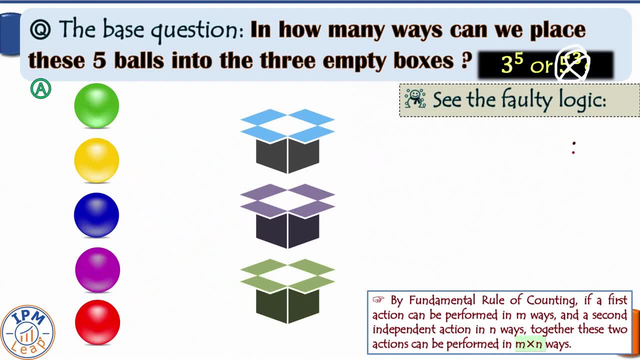 and means multiply. So our answer is: 3 raised power of 5.. By the way, if we had started with boxes- and try to see where this thought process goes wrong when you say box 1 can receive balls in 5 ways, that itself is wrong, because if we had to place 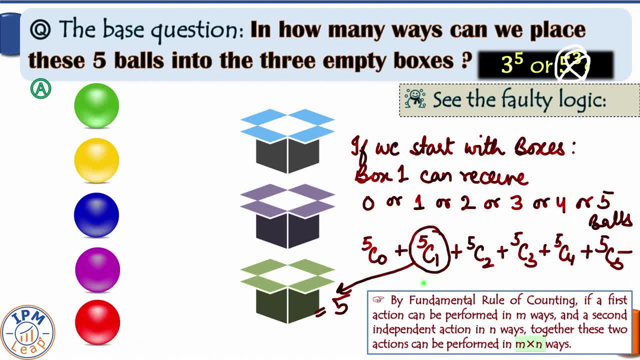 any one ball into it, it would be 5c1, that is, 5 ways. In that case, placing any two balls would be 5c2, that is, 10 additional ways. There are a total of 2 raised power, 5 ways, in which the first: 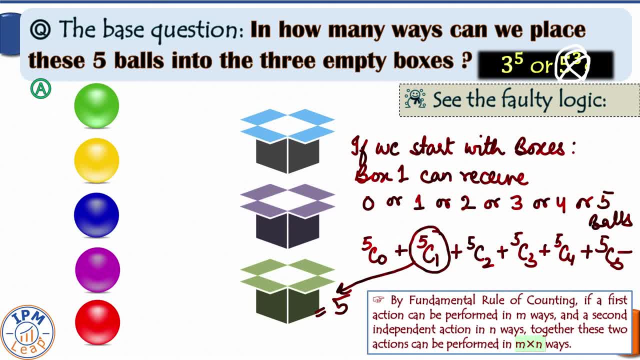 box can receive balls, but that's a topic for some other video. So let's get back to our question. Number of ways box 1 can receive balls is not 5.. Furthermore, depending on how many balls we place in box 1, the number of ways of placing balls in box 2 would change. So 5 raised power of 3.. 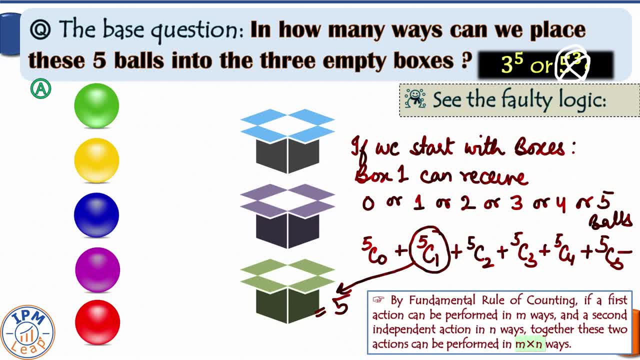 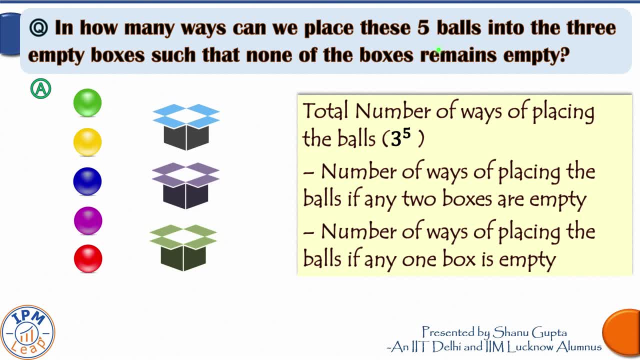 This option is incorrect. Now we come to our main question: In how many ways can we place these 5 balls into the 3 empty boxes such that none of the boxes remains empty? It's possible that when we are placing these balls into the boxes, all balls might go into any one box, leaving the other 2 empty. Another possibility: 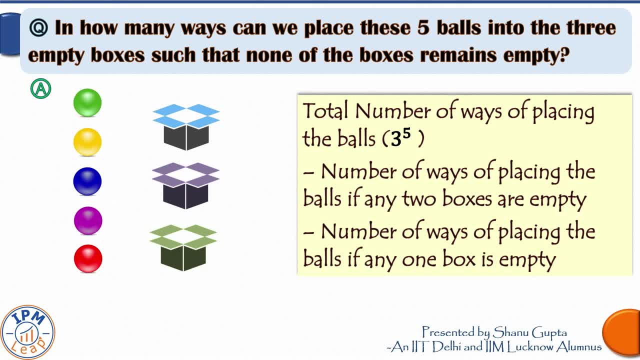 is that all 5 balls might together occupy any 2 boxes out of these, leaving the third empty. Like this is one possible scenario: The green, purple and red ball into box 1, yellow and blue in box 3 and box number 2 left empty. So, guys, our approach to solve this question is going to be very simple. 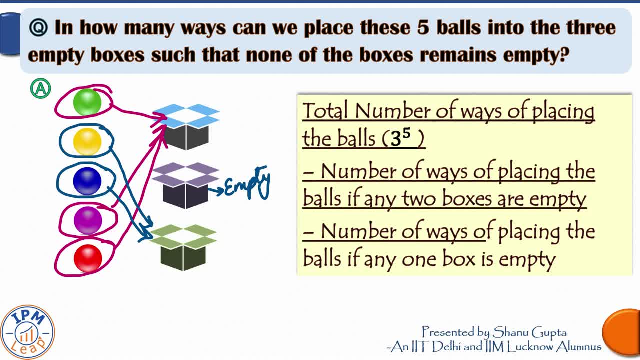 We just calculate the total number of ways of placing these balls. We just did that. they are 3 raised power of 5.. Out of these, if we subtract the number of ways of placing the balls where any 2 boxes are empty, or even any 1 box is empty, then we achieve our objective, isn't it? 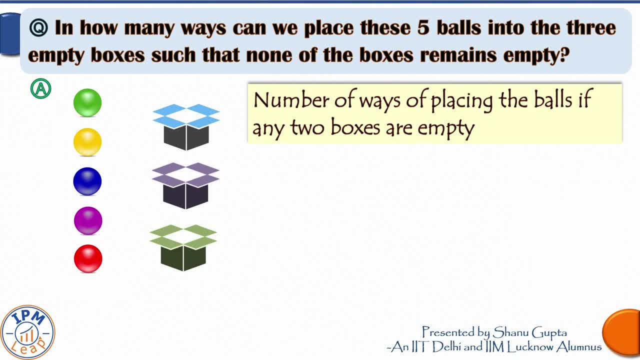 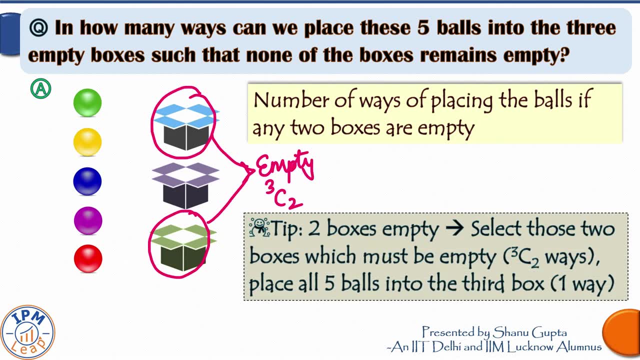 So what is the number of ways of placing the balls if any 2 boxes are empty? Very simply, we first select the 2 boxes which are left empty- 3 see 2 ways of doing that. Then all 5 balls must be placed in the remaining or the third box, which can be done in only 1 box. 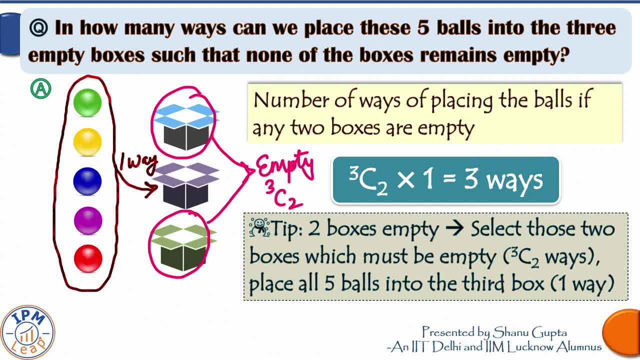 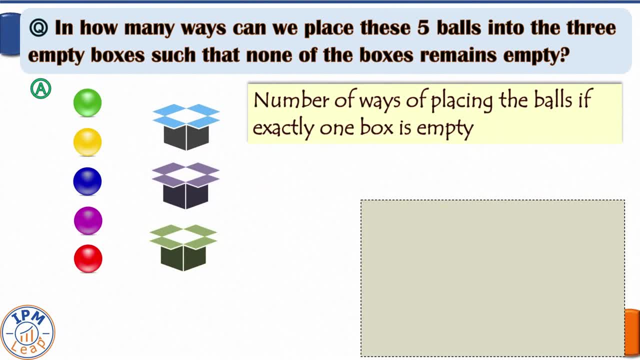 Hence, there would be 3 ways of placing the balls if any 2 boxes remain empty. Similarly, what is the number of ways of placing the balls if any 1 box is left empty? So, guys, first we select that box which should be empty. This can be done in 3, see 1 ways. 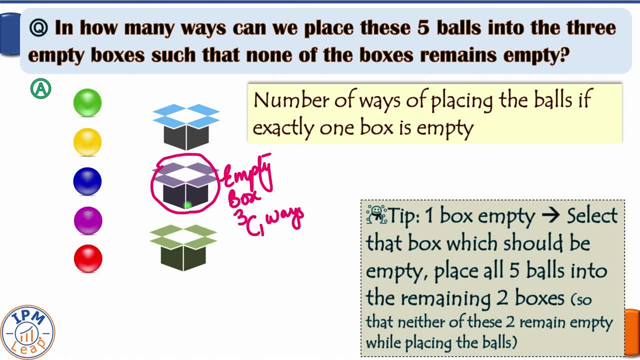 Say: this one is empty. Now all 5 balls are essentially placed into these 2 boxes, So we go through the whole process all over again. The first ball can be placed in 2 ways Correspondingly. the second ball can also. 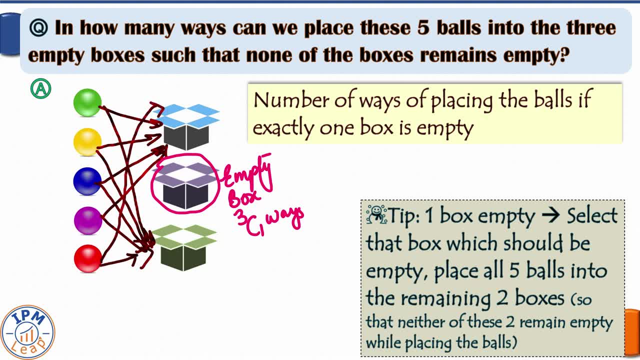 be placed in 2 ways, 2 ways for each ball. So total 2 raised power of 5 ways of placing all balls together. But a word of caution: Out of these 2 raised power, 5 ways, we must make sure. 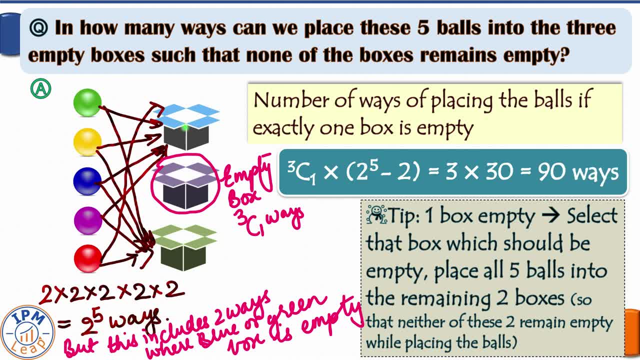 that none of these 2 boxes remain empty this time, Because that would mean a total of 2 boxes go empty instead of 1.. We have already taken that number into account. Well, if all 5 balls go into either this box or into this box, then the other box goes empty. That is 2 cases out of these. 2 raised power 5. 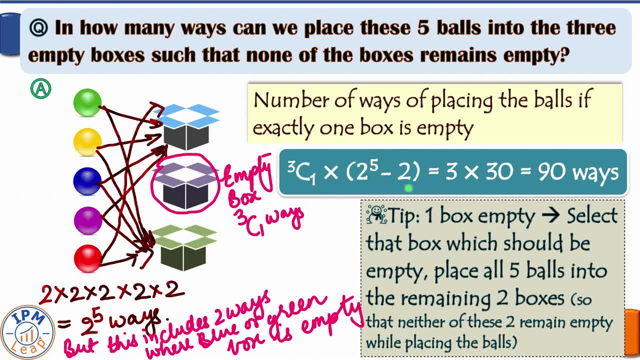 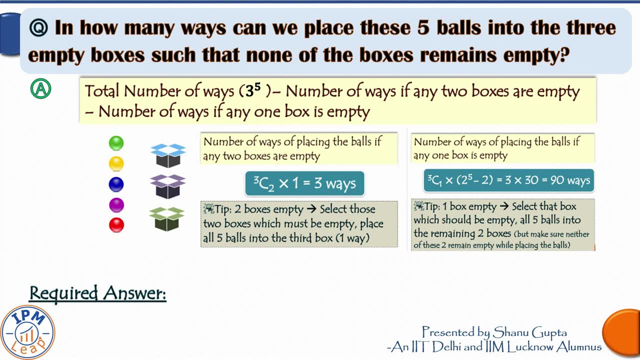 cases we need to subtract: This is equal to 3 and this is 30. So there are 90 ways of placing the balls if exactly one box goes empty. To find out our answer, we subtract the numbers for these 2 cases from the total 3 raised power: 5 minus 3 minus 90.. 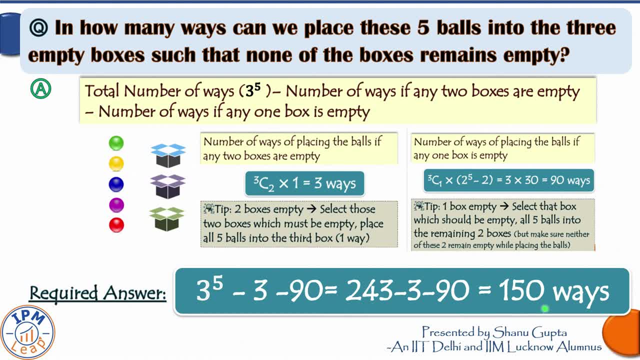 243 minus 3 minus 90. This calculates to 150 ways- And that is our answer: 150 ways- of placing these 5 balls into the 3 raised power 5 boxes. This is equal to 150 ways of placing these 5 balls into the. 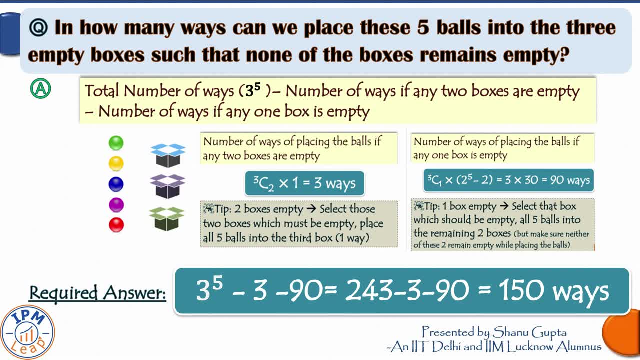 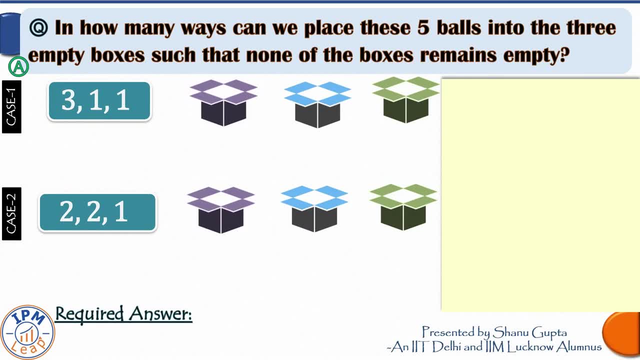 3 empty boxes, such that none of the boxes remains empty. The same question can also be solved by grouping the 5 balls into 3 lots. See, there are only 2 possibilities: These 2.. Either we have 3 balls going into one of the boxes. 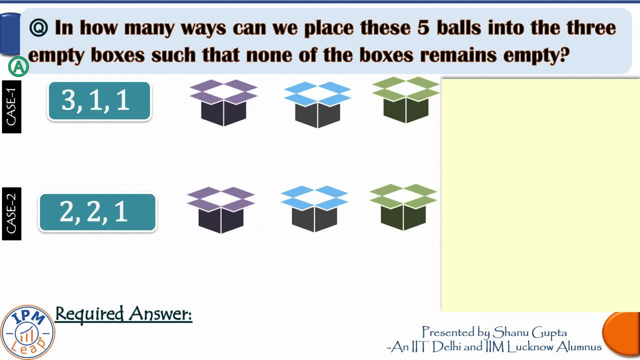 and 1 each in the remaining 2.. Else, we have 2 balls in one of the boxes, 2 in some other and the remaining ball in the 3rd box. In these 2 ways of placing the balls, a required condition- that none of the boxes remains empty- holds true. 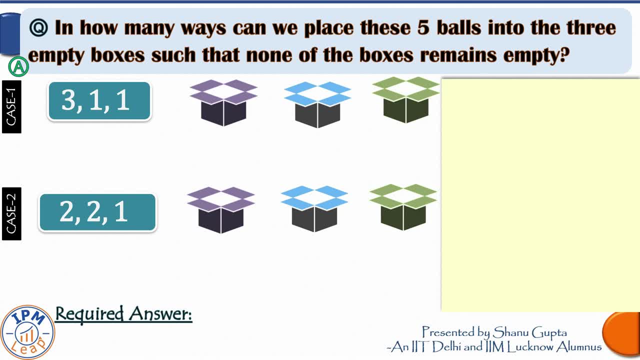 We just need to count the numbers for each case. So for case number 1, we first select the box which receives 3 balls. One box out of 3 can be selected in 3 ways. next, we select the three balls out of the five given balls to go into that box. three out of five.